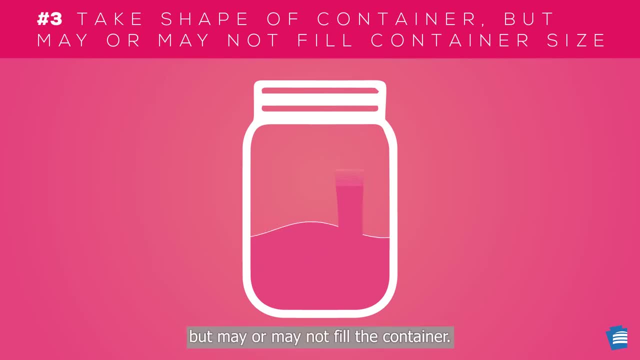 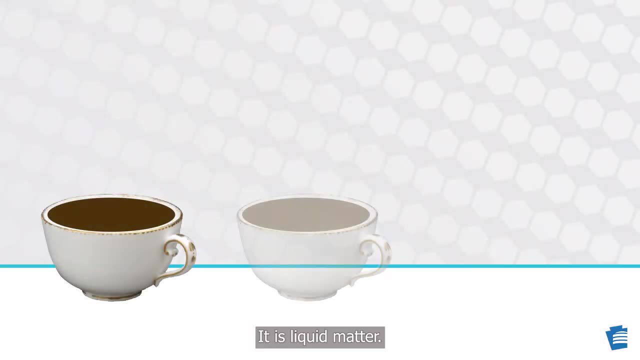 will take the shape of the new container, but may or may not fill the container. Let's look at my tea. It is liquid matter. If I have three identical cups of tea with the same amount of tea in each cup, does the tea take the shape of the new container? 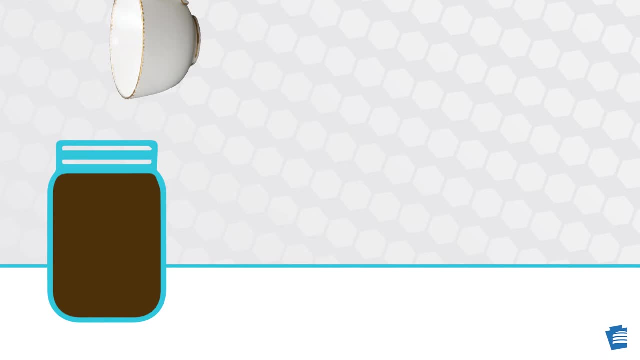 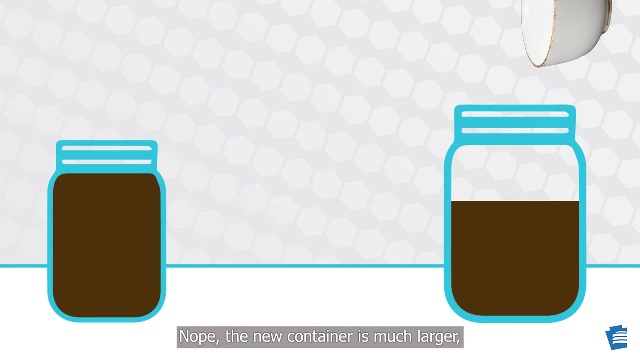 Yes, Liquids can change shape, but it's still the same amount of tea. The tiny particles just shifted their positions within the shape of the tea. Does the tea fill the container? Nope, The new container is much larger, so the tea took the shape of the container but didn't fill it. 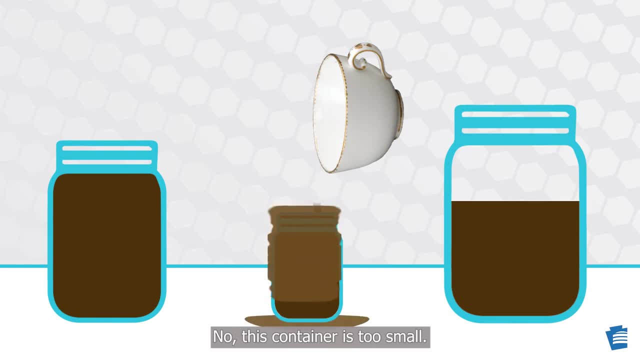 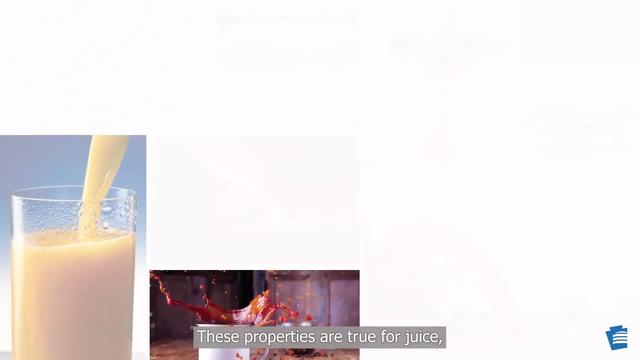 Does the tea fit Into the new container? No, This container is too small. Can I squish or compress more tea into the container? Nope, It just overflows the container. These properties are true for juice, honey, paint and many other things. 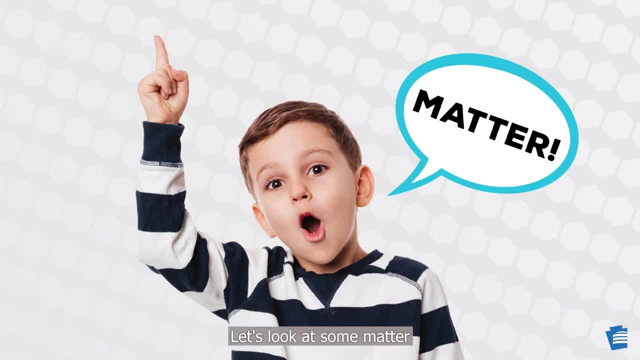 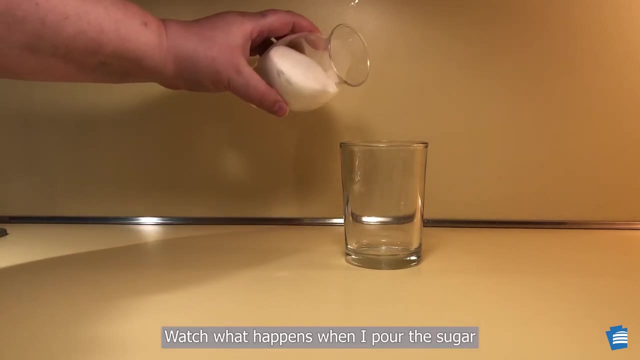 These are all liquid. Let's look at some matter and see if we can decide if they are liquids. OK, Put on your thinking cap. This is sugar. Is sugar a liquid? Watch what happens when I pour the sugar into a new container. 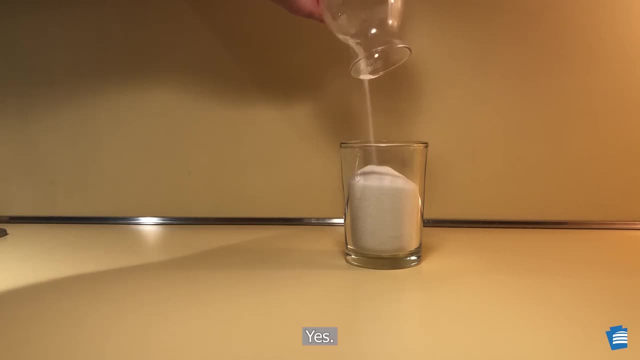 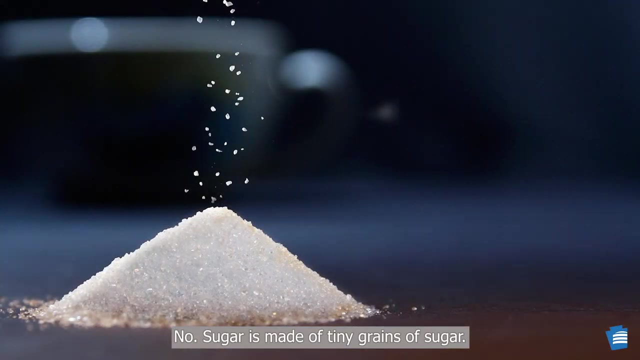 Does the sugar flow when I pour it? Yes, Does the sugar take the shape of the new container but not fill it? Yes, Is sugar a liquid? No, Sugar is made of tiny grains of sugar. The grains flow or slip past each other, adjusting their positions as they fill the new container. 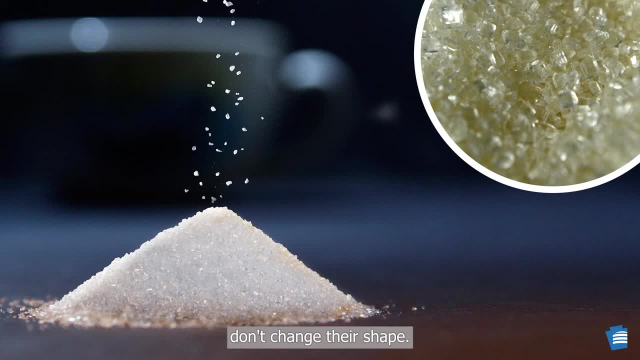 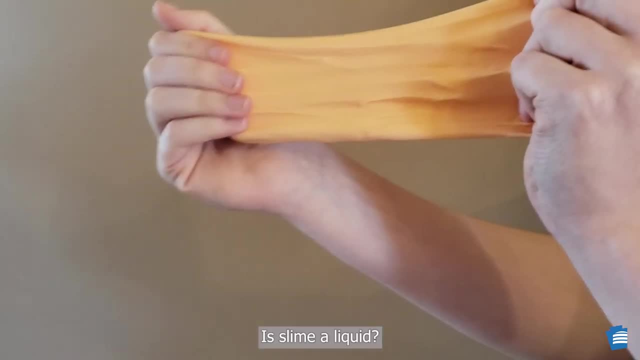 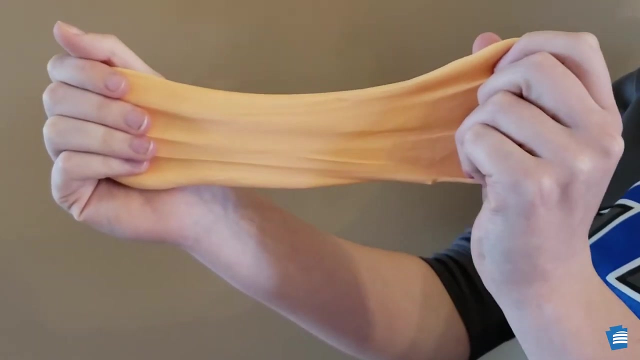 But the actual grains of sugar don't change their shape. Sugar is a solid. Let's look at slime. Is slime a liquid? Can the slime change shape? Yes, When the slime changes shape, it's a liquid. When the slime changes shape, do we get more slime?